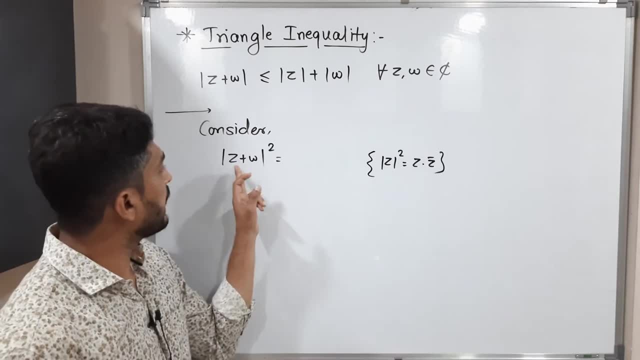 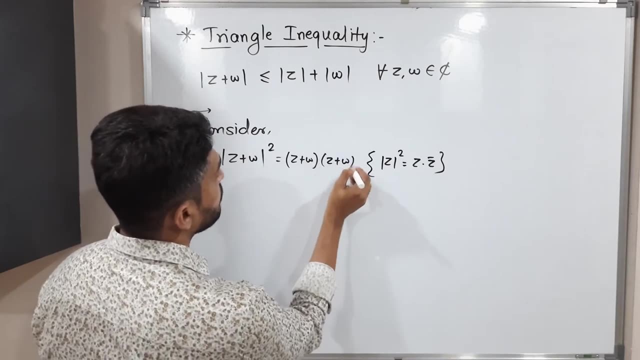 this result here. What can we write At a place of z? we have z plus w, Okay, so by using this result, we can write z plus w, z plus w bar, Okay. so we are using this result here. So this is equal to. 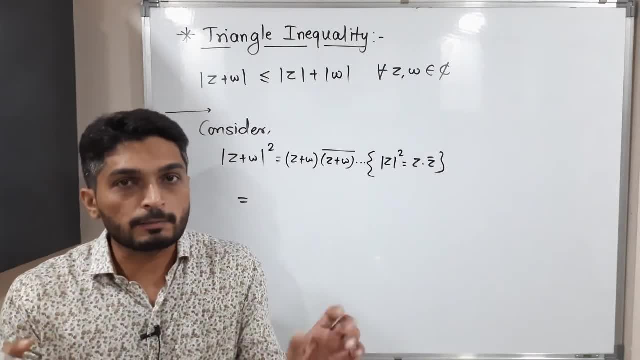 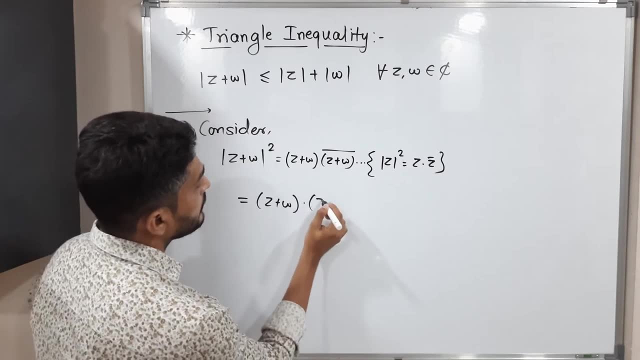 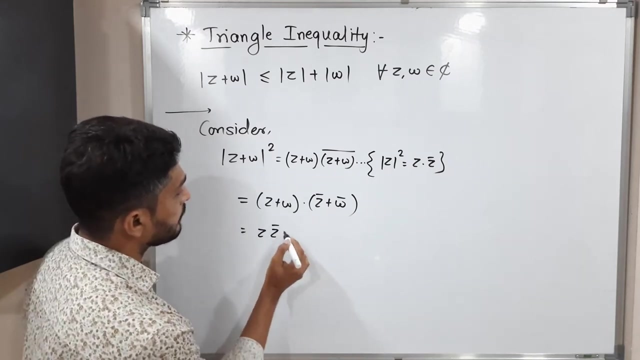 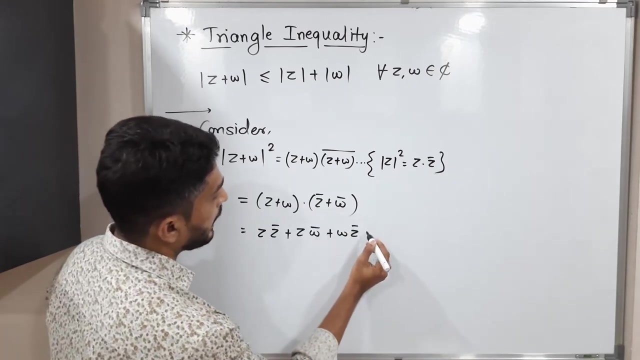 So you know that if addition is there, definitely we can take separate, separate bar. okay, that means it's complex conjugate, so we can write z plus w into z bar plus w bar. let us take product. so first into first. that means z into z bar plus z into w. that means z into w bar plus w into z bar. right and plus. 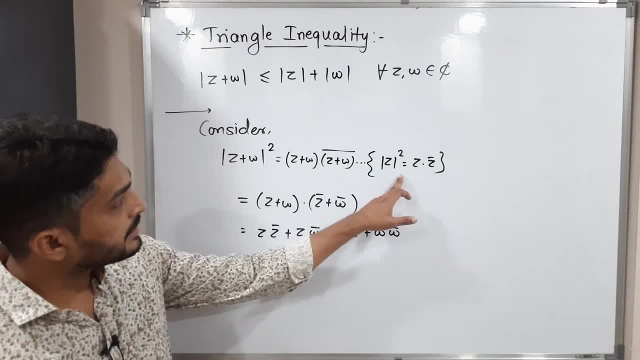 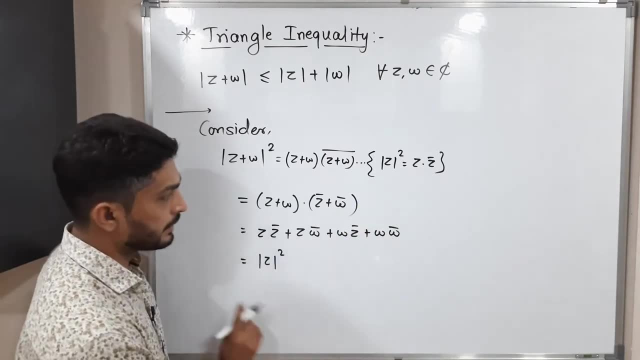 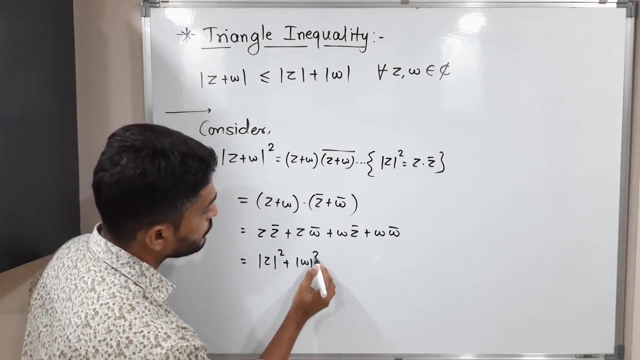 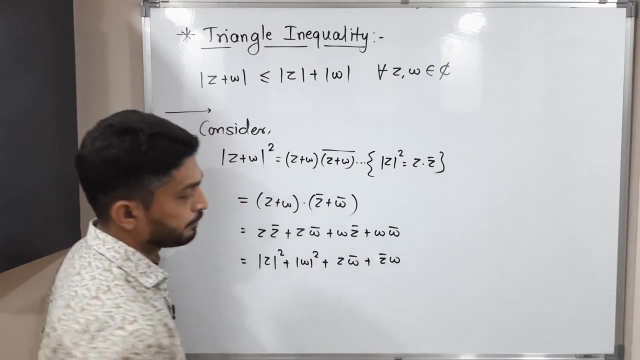 w into w bar. let us use this result again here. okay, z into z bar means what mod z square, so we can replace it by mod z square. similarly, for this term also w into w bar. so using same result, we can write mod w square. so, plus what we have, z w bar, right, plus i will say z bar w. okay, so see now. 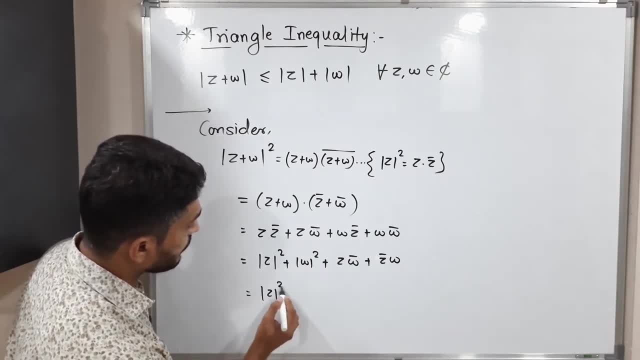 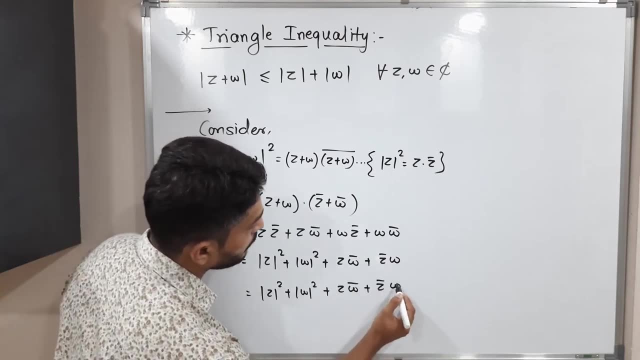 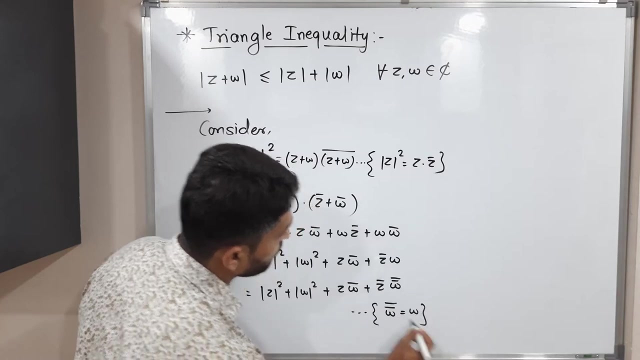 what will i do? so? this is equal to mod z square plus mod w square plus z w bar plus z bar w bar w bar, since we know one result that is w bar bar is nothing but w. so if you take complex conjugate of complex conjugate, you will have the 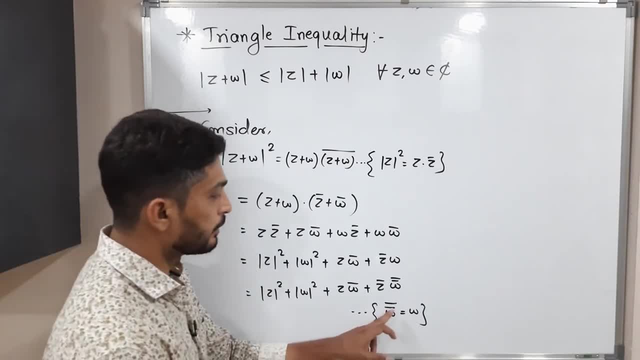 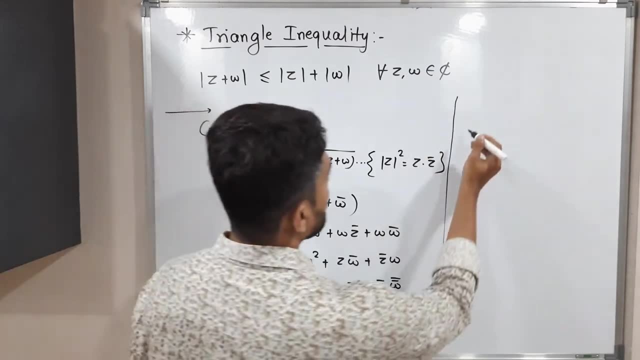 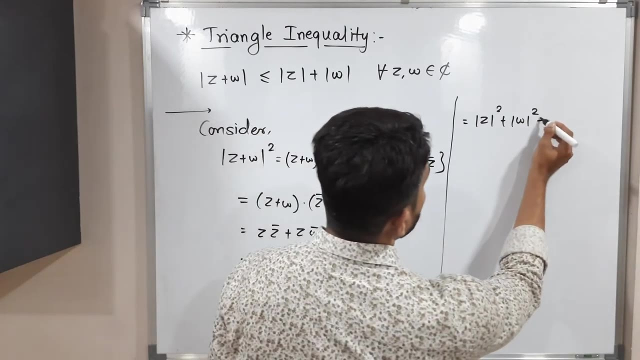 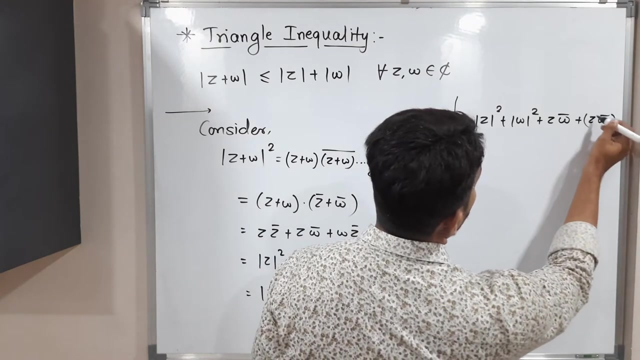 original complex number. so the same thing here. so that's why w w bar is equal to w. so that's. i replace w by w double bar. okay, so let me continue here. this is equal to what we have: mod z square plus mod w square. okay, so plus z w bar right, plus z w bar whole bar. okay, so z has one. 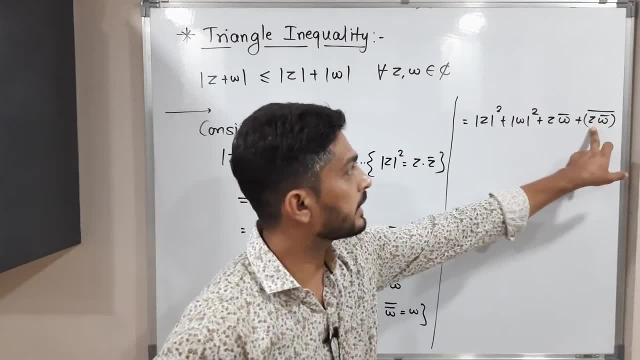 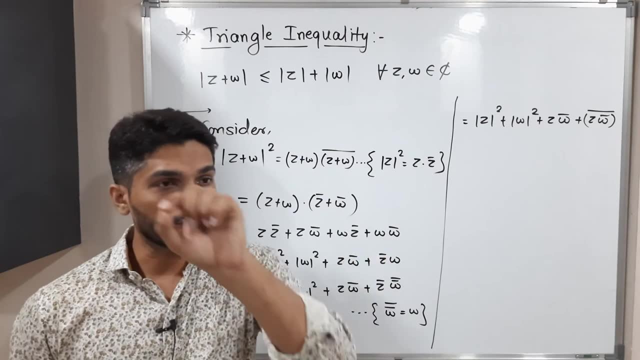 bar. w has double bar, so i can take one bar common and we can write z w bar, since you know that z, that means if you have a product of two complex number, z and w, if you write bar you can take separate, separate bar. okay, so using that result, i could write it. so is equal to what can we write? 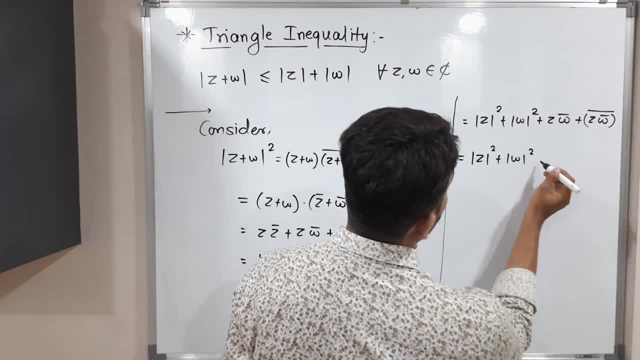 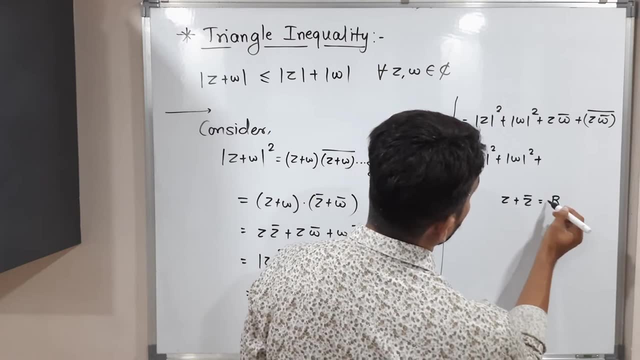 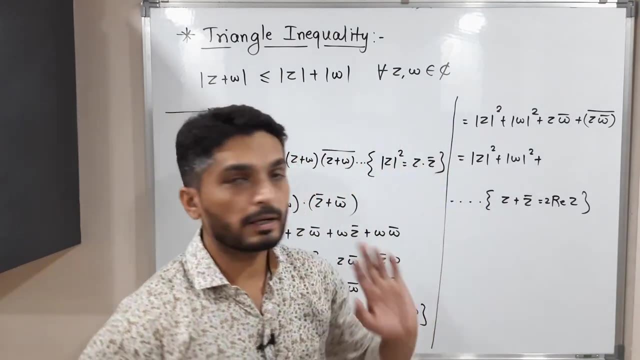 mod z square plus mod w square plus. okay, so let me tell you one thing, that is, a z plus z bar is equal to 2 into real part of z. so this result we have already seen. okay, z plus z bar is equal to 2 into real part of z. either we have seen, i think, in 11 standard, 12 standard or in bsc also we have 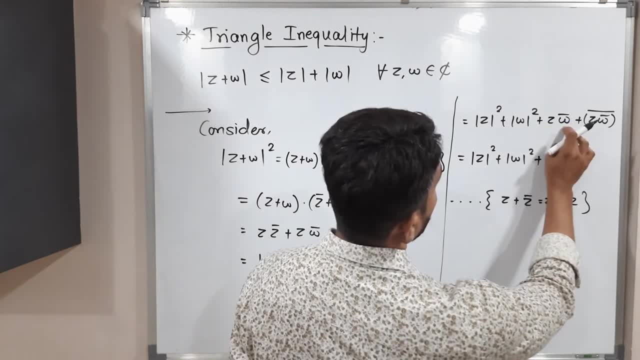 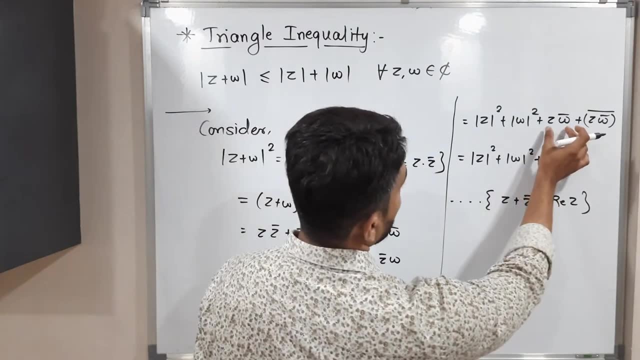 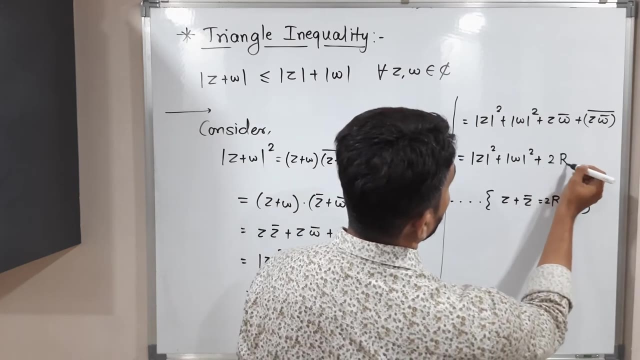 seen right? so see, both complex number are same: z w bar. here also we have z w bar, just we have one additional bar there, right? so if you consider z w bar by z, so we have a same type of relation. so this is equal to 2 into real part of z, so we can write 2 into real part of z w bar. okay, using this result, i can write: 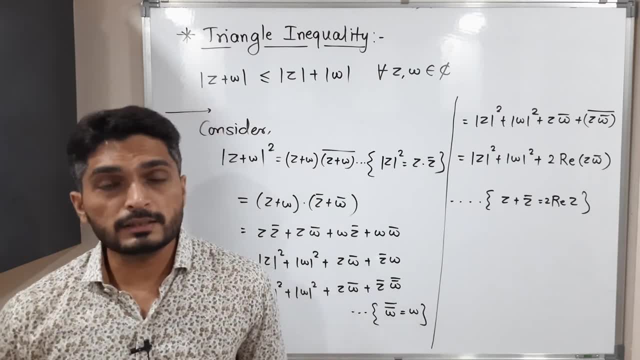 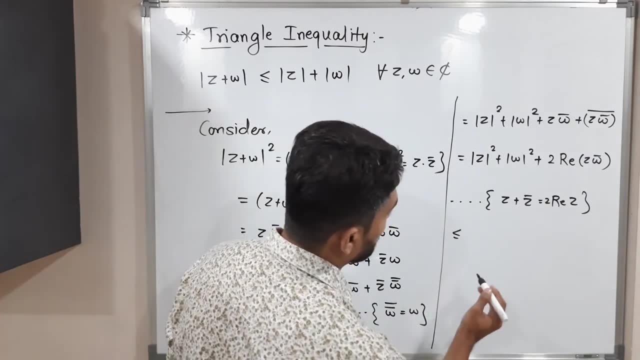 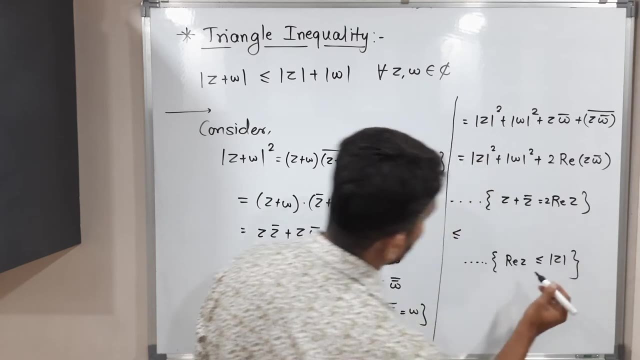 it. but see, we know that real part of any complex number is always less than or equal to modulus of that complex number. okay, so using that result, i can write less than or equal to. let me mention the result first here. so that result is real part of z is always less than or equal to mod z. okay, so, using this result, what can i write here? i am 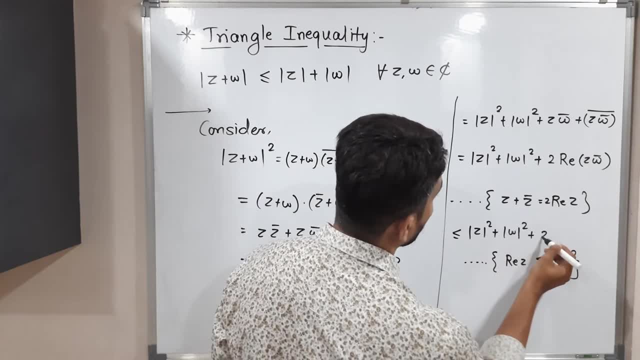 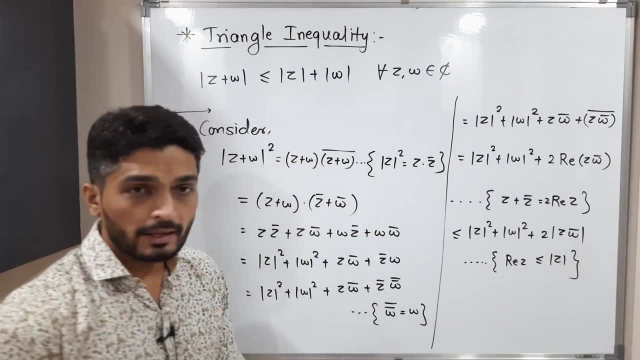 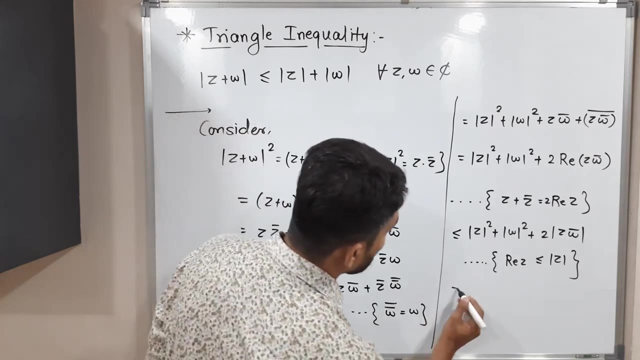 writing mod z square as it is. mod w square as it is plus 2, real part of this one is less than or equal to mod z w bar. we have seen in a property of mod. if you have a product you can take separate, separate mod. so let me write it here: so this is equal to mod z square plus 2 into real part of z. 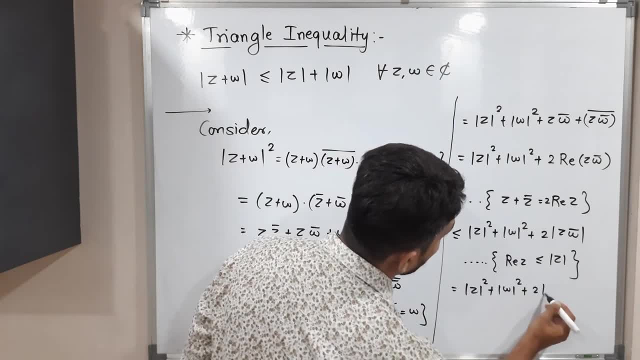 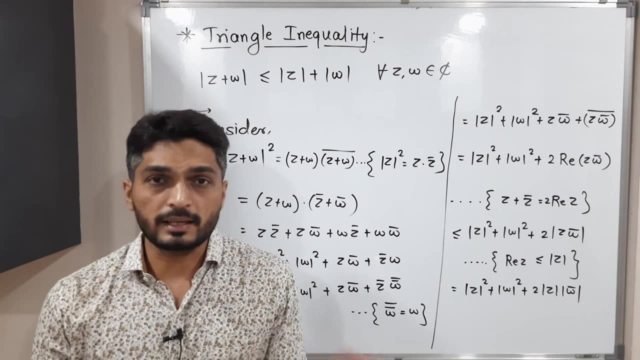 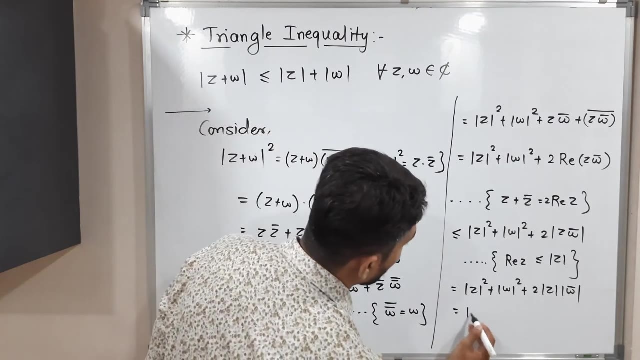 square, plus mod w square, plus 2 mod z, mod w bar, but see mod of w and mod of w bar. both of them is same, getting so already we have seen that thing. mod z is same as mod z bar, so that's why we can write here: so this is equal to mod z square. see all these properties we have already seen simply. 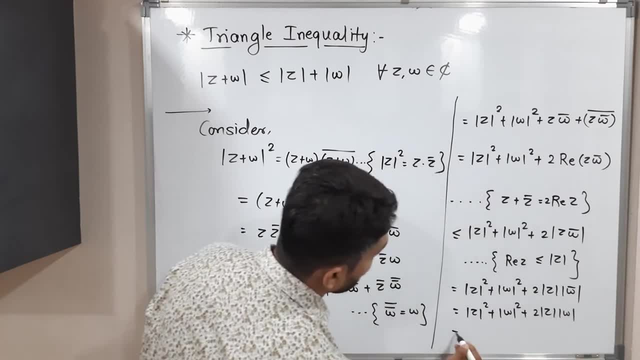 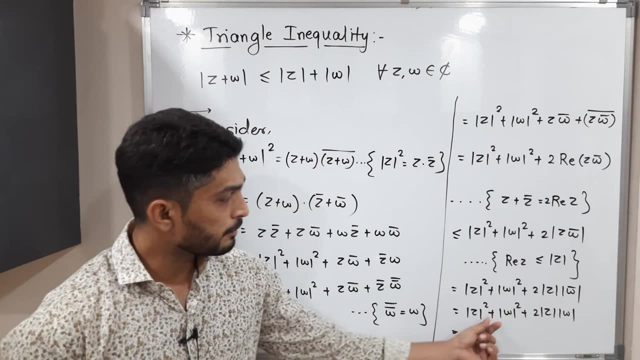 we are using the properties which we have already seen. okay, so what can we write? okay, can we use any formula here? have you seen such type of equation anywhere? mod z square, mod w square plus 2 into mod z mod w. so this is simply bracket square formula: a plus b.